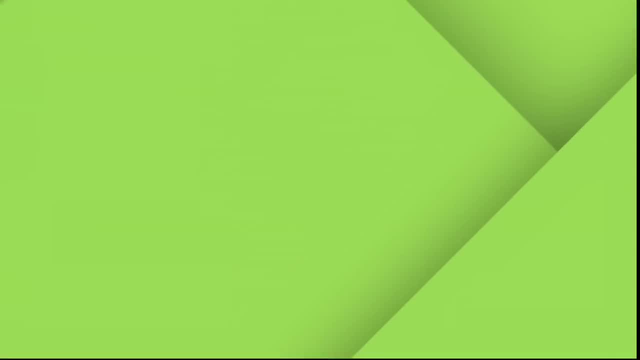 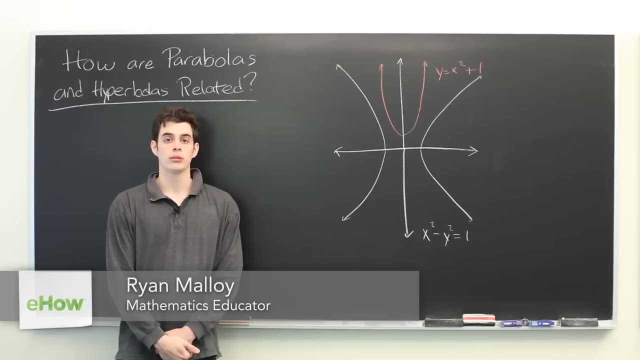 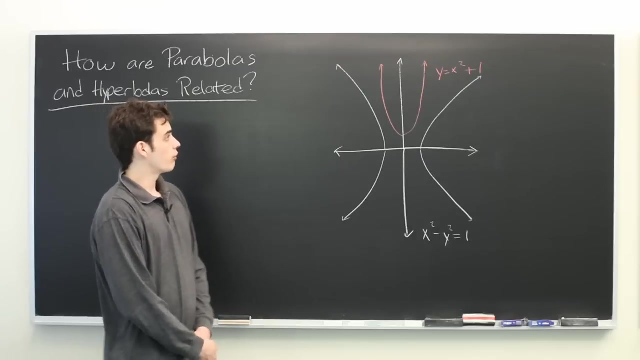 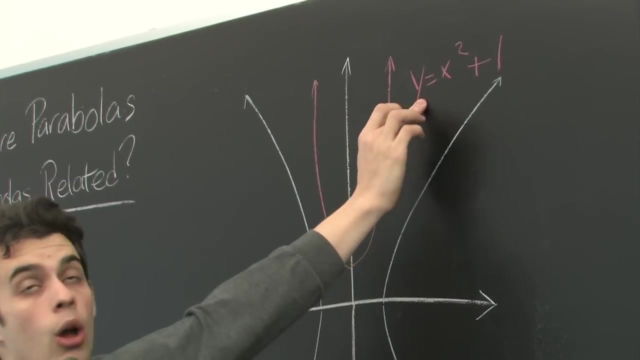 Hi there, This is Ryan Malloy here at the Worldwide Center of Mathematics. In this video we're going to discuss how are parabolas and hyperbolas related? To quickly review what those two terms mean, here we have a parabola that is defined by the equation y equals x squared. 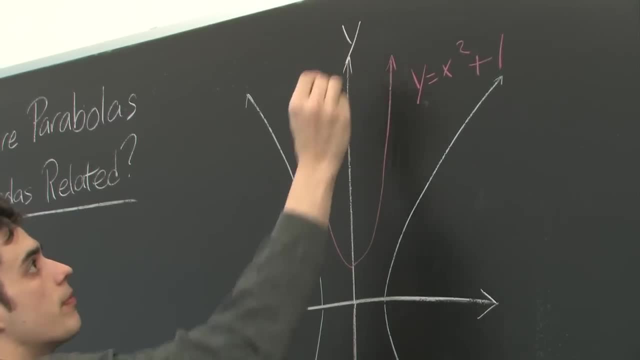 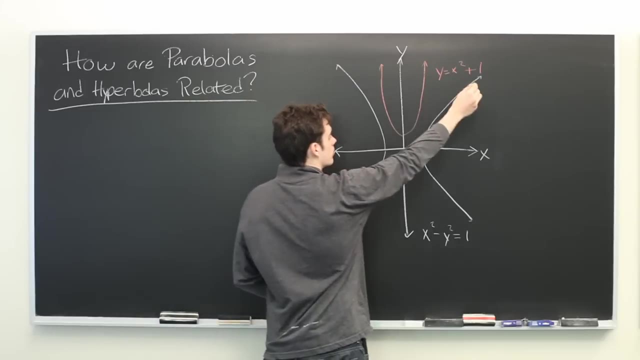 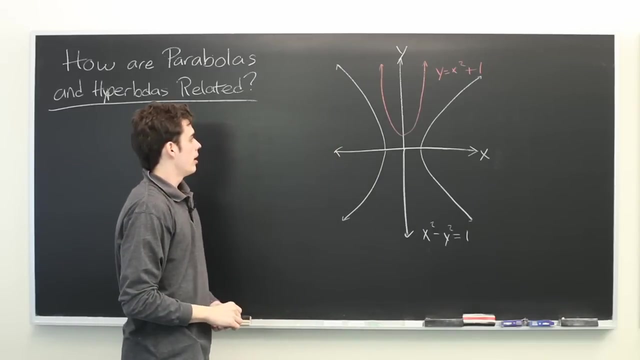 plus 1.. Here we have our y-axis and here we have our x-axis. The two blue curves are generated by this equation: x squared minus y squared equals 1.. And while they're both curves, it might not appear that they're related in any interesting way. After all, this one. 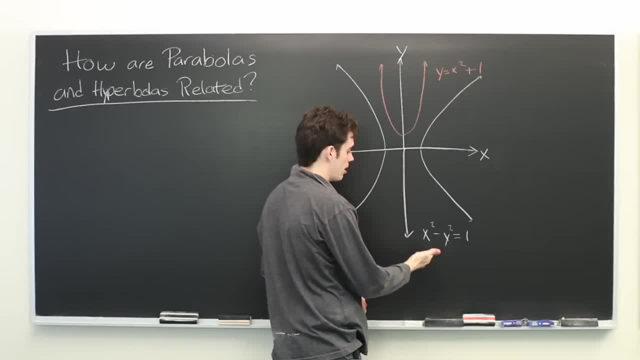 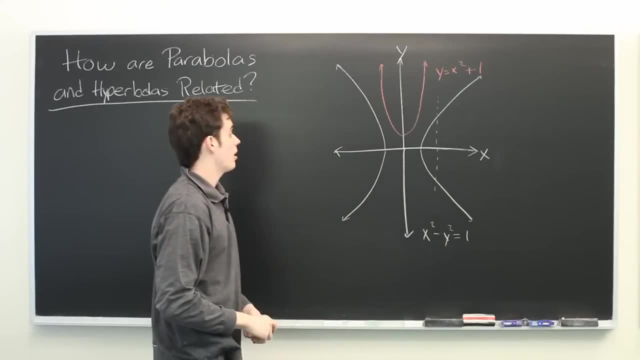 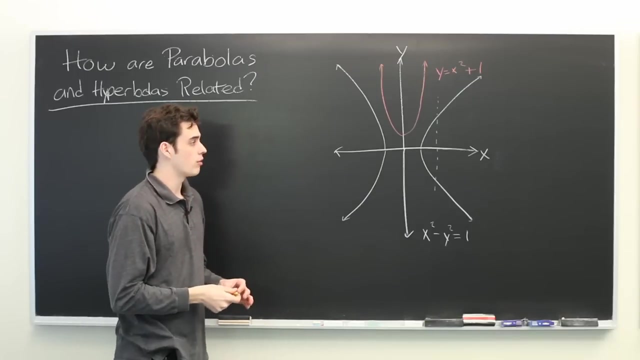 is a function that is explicitly defined and this is not a function. You can see it does not pass the equation, The vertical line test. So it might not appear that there is any real relation between them, But both of these types of curves are examples of what we like to call conic sections. If 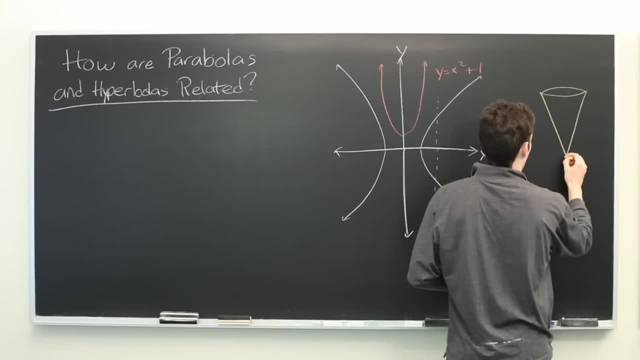 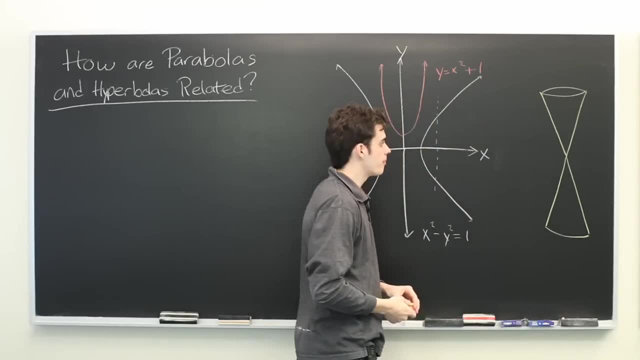 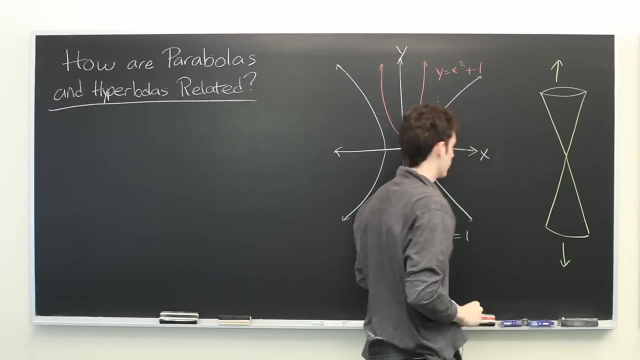 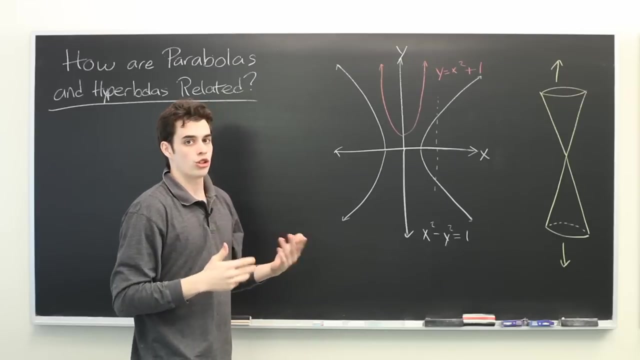 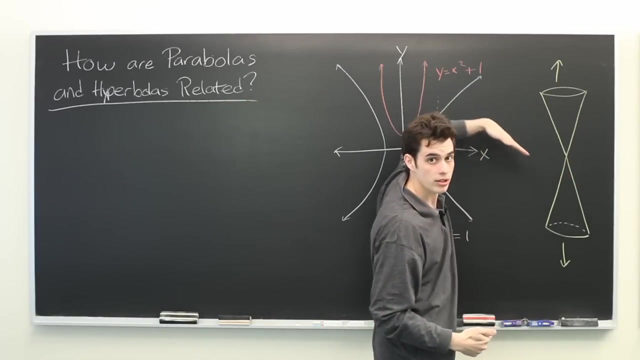 you were to draw a cone that is stacked on top of itself, in a sense that extends the cone outwards towards infinity, both above and below. you can create a few different shapes by taking sections of the cone. If you imagine chopping the cone into two parts. 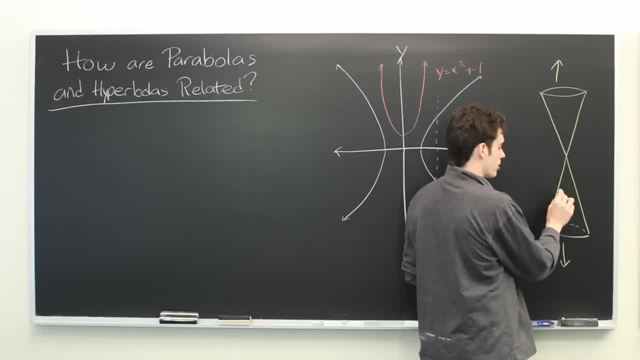 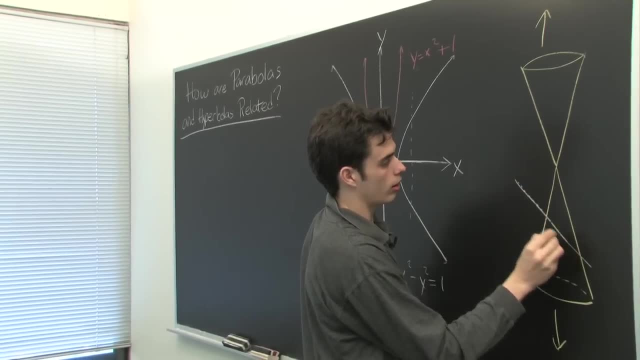 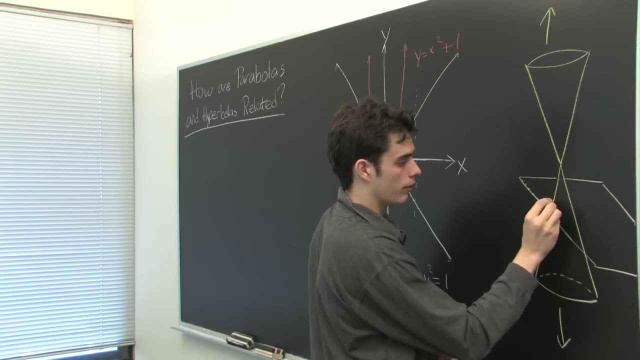 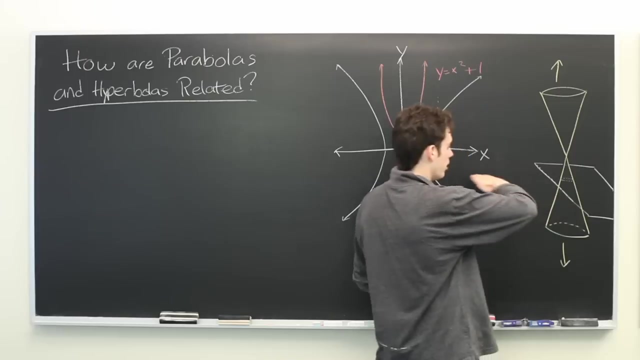 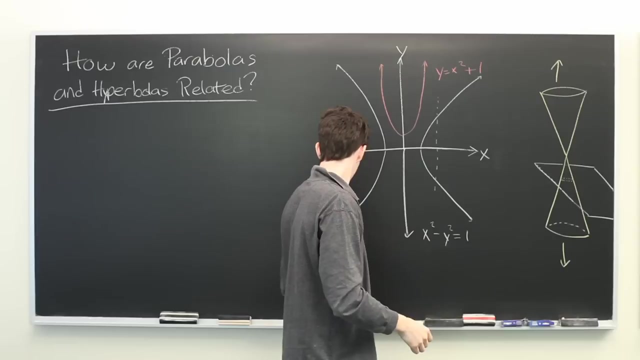 using a plane. the set of points that the plane intersects with the cone will create a conic section. So, for example, here take this white plane that cuts directly across the cone- you�ll get a conic section. that's simply a circle.